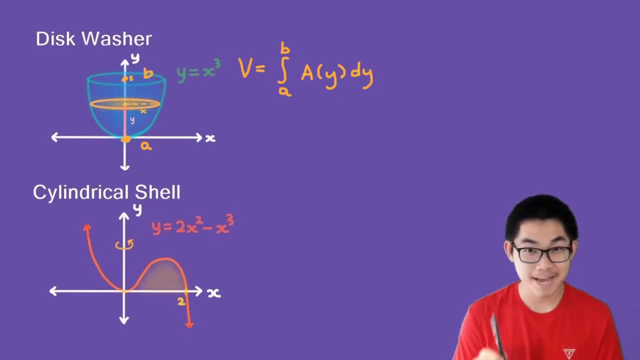 let's go ahead and find the volume so step number one we want to find a and b so since a is right here at the center then a is equal to zero where b is equal to eight so i wrote the number eight right there so b is going to be equal to eight 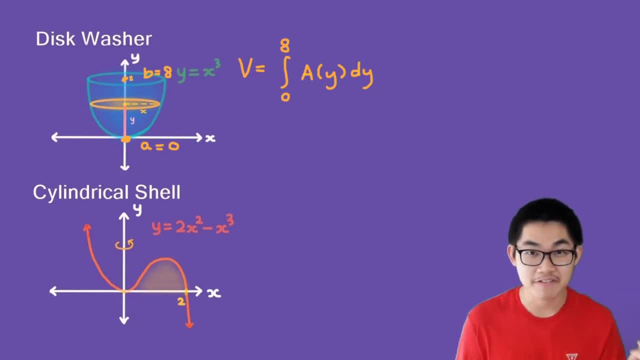 step number two is to find the area of the cross section so since the cross section or the dish is a circle then the area must be pi times the radius to the power of two so the area a of y is equal to pi times the radius to the power of two so since the cross section is equal to two now the distance from the center until we reach the 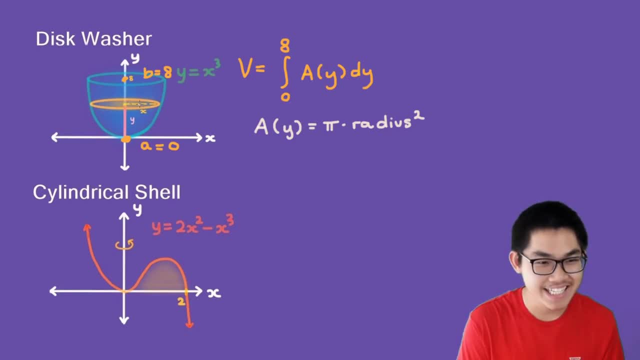 cross section is y and the distance from the y-axis until we touch this function this distance is x and so the radius is x so the area is the same as pi times x to the power of two 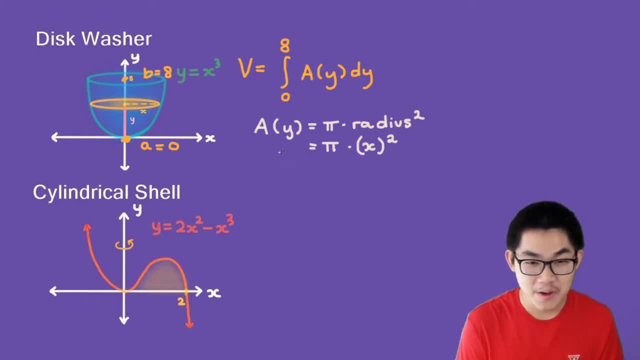 so since we're trying to integrate with respect to y we need to rewrite this function in terms of y now we know that y is equal to x to the power of 3 so if we take the cube root of both sides we're going to get x is equal to y to the power of 1 3 and we can replace it with x right here so finally the area is equal to pi times y to the power of one third 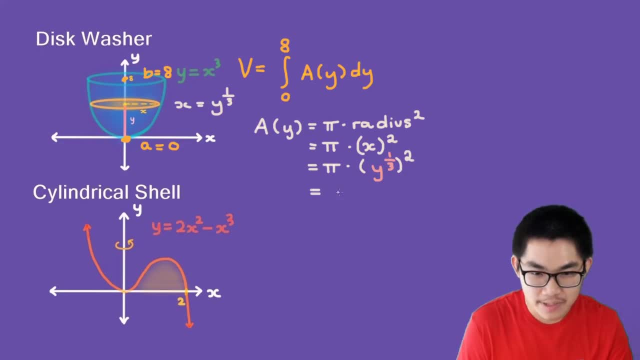 to the power of 2, and that will simply give us pi times y to the power of 2 thirds. 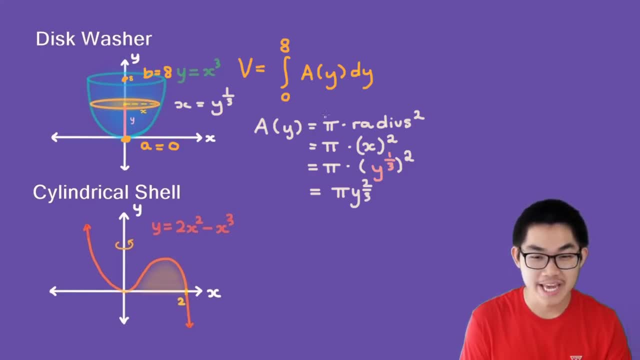 Now we found the area of the cross-section, we can go ahead and substitute it back into the integral. 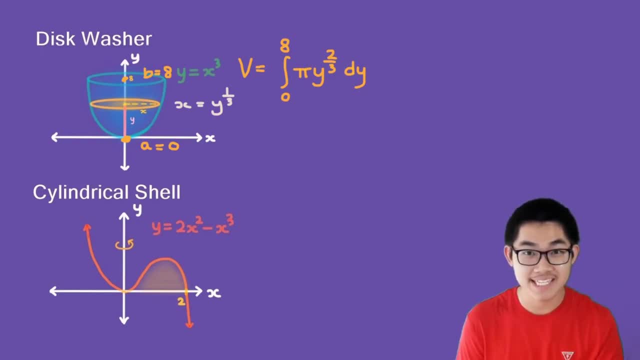 The third and final step is to evaluate this integral. So since pi is just a constant, we can move it outside of the integral. So v is equal to pi times the integral from 0 to 8 of y to the power of 2 over 3 dy. 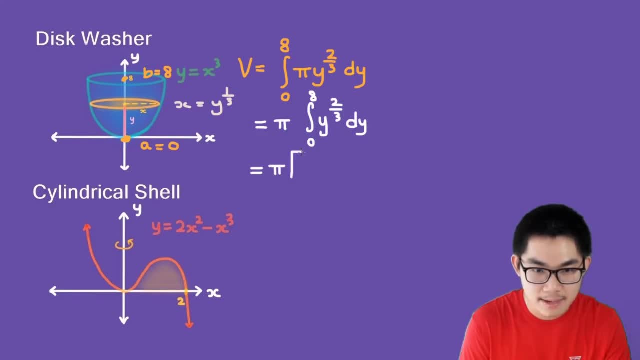 This is the same as pi times the antiderivative of y to the power of 2 over 3. So we're going to get y to the power of 5 over 3, and then we divide by 5. So when you divide by a fraction, it's the same thing as multiplying by its reciprocal. And then the limit goes from 8 to 0. 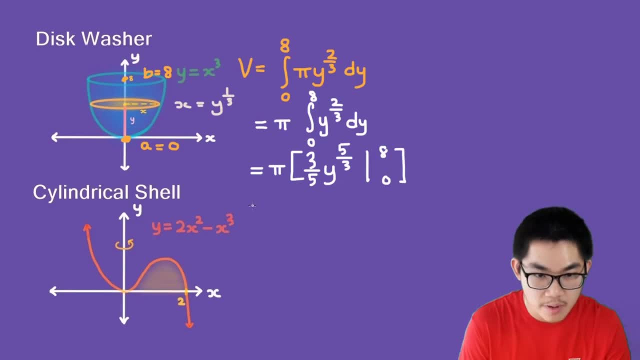 So the next step is just substituting these numbers into our formula. We're going to get pi times 3 over 5 times 8 to the power of 5 over 3, minus 3 over 5 times 0 to the power of 3. 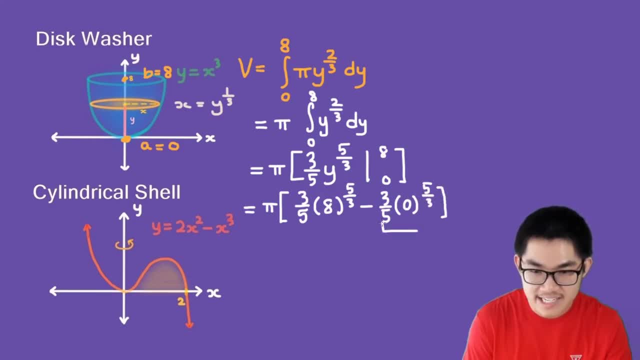 So we know right away this right here is going to be 0. 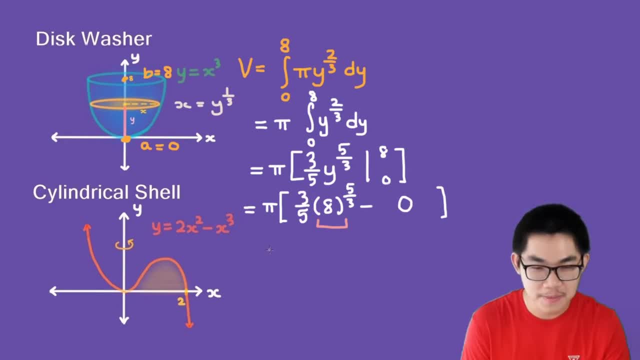 Now, what is 8 to the power of 5 over 3? Well, 8 to the power of 5 over 3 is the same as 8 to the power of 1 over 3 to the power of 5, which is the same as 2 to the power of 5, which is just 32. So pi times 32 times 3 is going to be 96 over 5. And the final answer is equal to 96 over 5 times pi. Now, you can leave it the way it is, or you can say union to the power of 3. Basically, that means we have found the volume of this 3-dimensional shape using the dishwasher method. 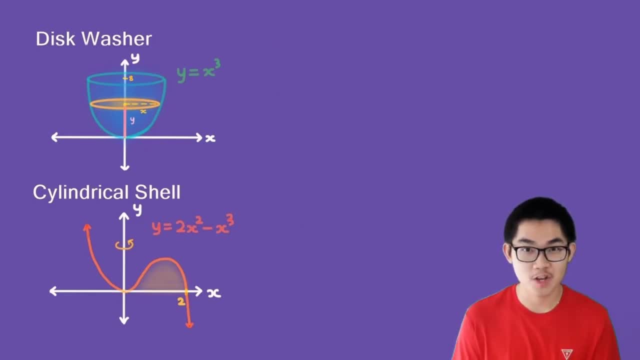 Now, let's take a look at the second method to find the volume, which is the cylindrical shell method. 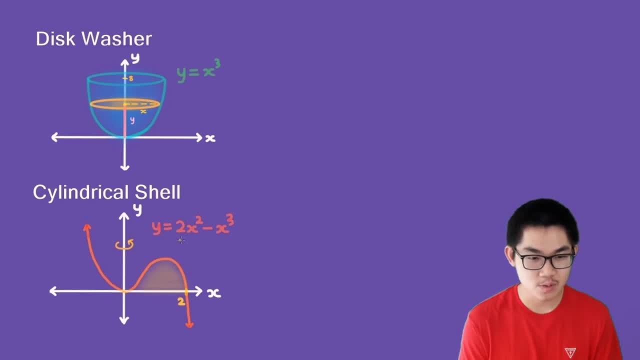 So we have a function y is equal to 2 times x to the power of 2 minus x to the power of 3. And we're going to take the area between this function and the x-axis and rotate it around the y-axis. 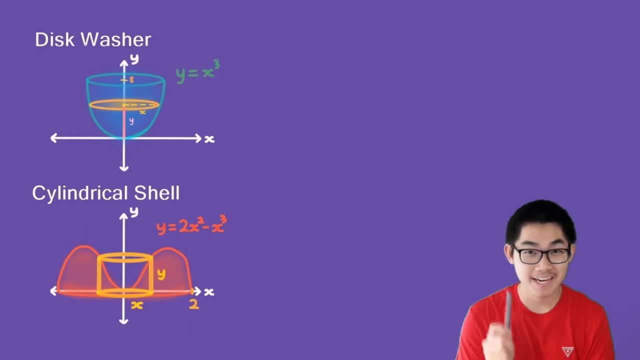 Before I show you how to find the volume, I would like you to pause the video and try finding the volume using the dishwasher method. 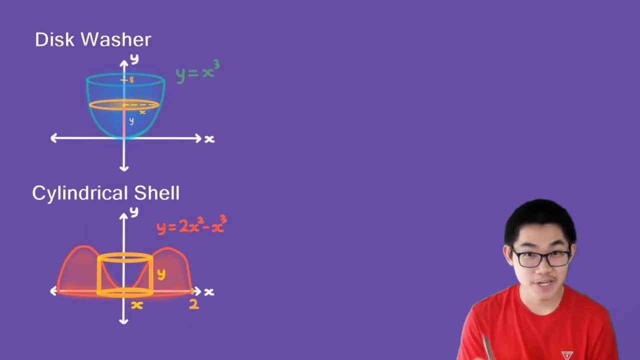 And you will notice that it's impossible. The trick here is if the shape that you get does not look like a cucumber cut in half. 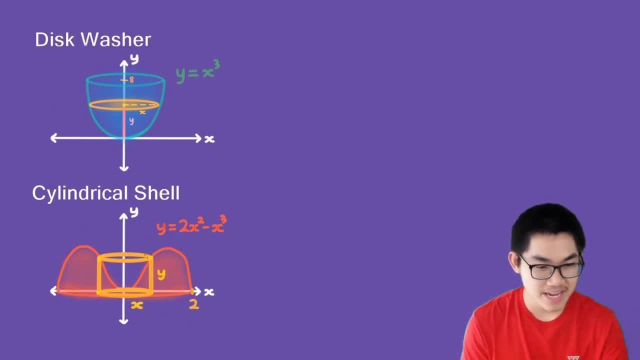 So in this case, our 3-dimensional object looks kind of like a mountain with a dent inside it. And it does not look like a cucumber shape cut in half. 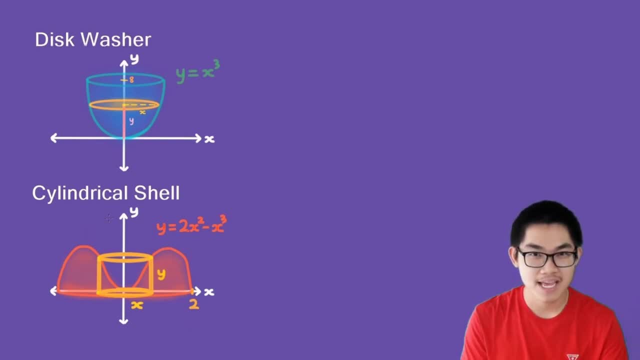 You have to use the cylindrical shell method. And the shell method says that if we have a cylinder, if we put the cylinder here, and the base of that cylinder is on the x-axis, then you integrate with respect to x. If the base of the cylinder is on the y-axis, so if the cylinder looks like this, and the base of the cylinder is on the y-axis, then we integrate with respect to y. In this case, it's on the x-axis. 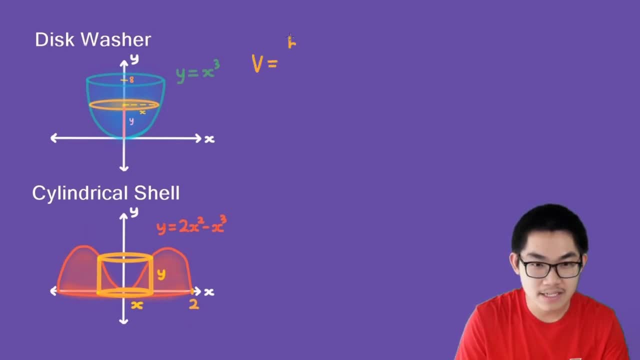 So the volume formula will simply be the integral from a to b of 2 times pi, times the radius, times the height. 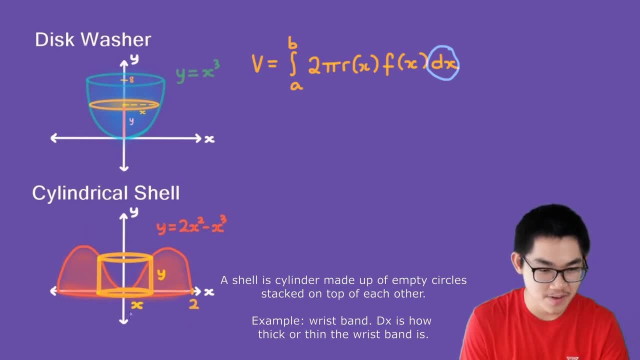 d of x is just the thickness of the shell. So it's basically the distance from here to here. That's going to be the thickness of the shell right there. 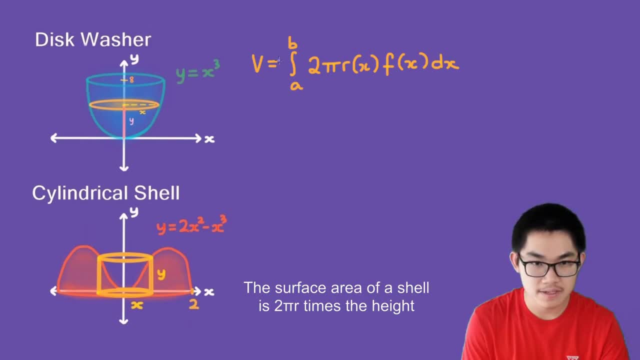 So what this formula is saying is from a to b, so from a right here, and b, this is a and that's b, we're gonna take the volume, we're gonna take the volume of each shell. 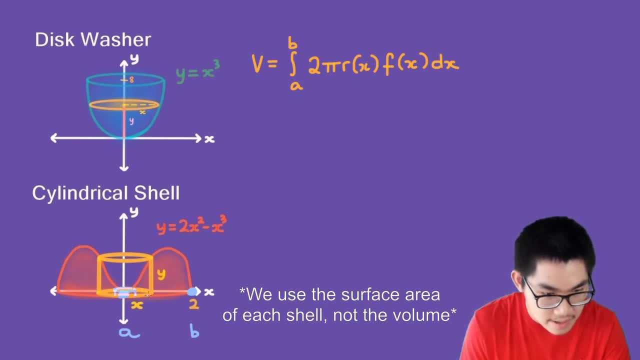 So we're gonna take the volume of this shell right there, 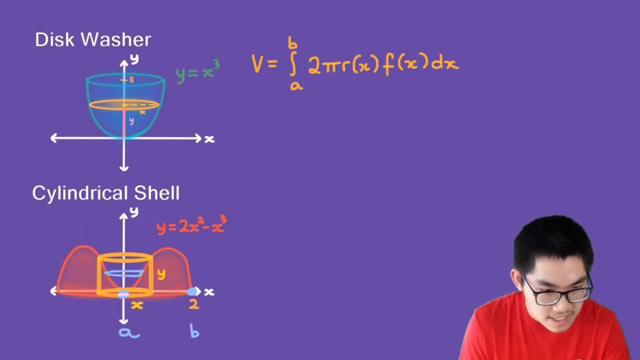 and then we're gonna take the volume of this shell, moving from here to here, right? So the volume of this shell, 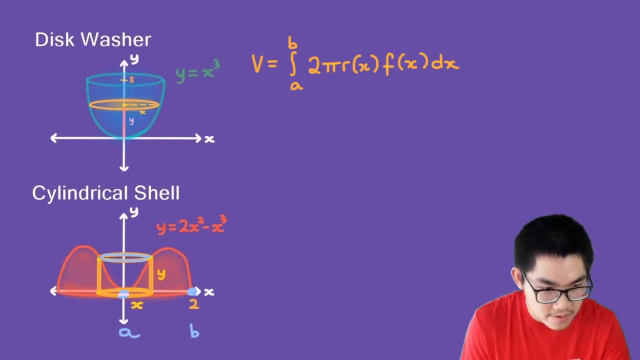 and then we're gonna take the volume of this shell right here, 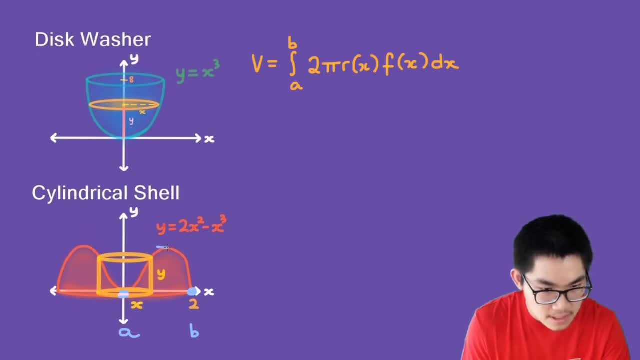 and then as we move towards b, we're gonna take the volume of this shell right there, and then we're gonna take the volume, of this shell, 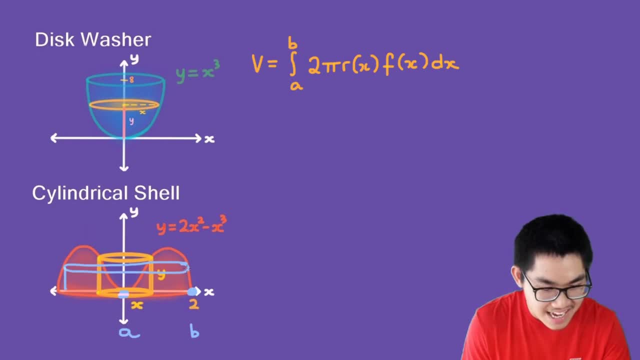 so I think you understand what I mean, and then finally we're just gonna take the volume of the final shell, so this shell right there. 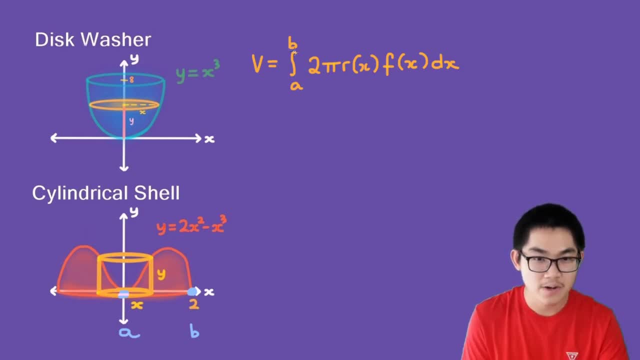 And the integral sign right here means that we add all of those volumes of our shells together, and that's going to give us the volume of our three-dimensional object. 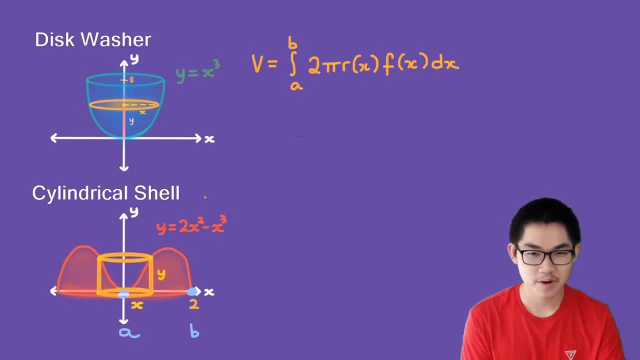 Now let's find the volume of this shape using the formula. So, step 1. 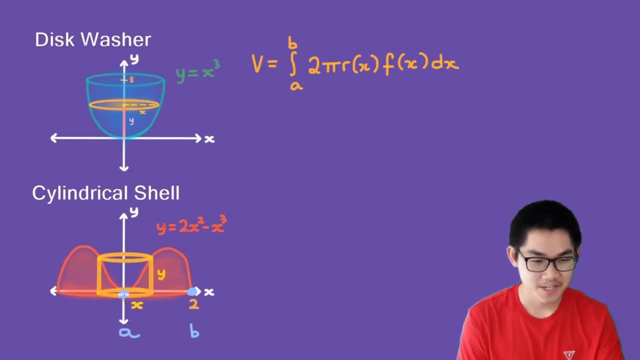 number one is to find a and b so a is going to be in the middle so a is at the center and therefore a is equal to zero and b is right here so b is equal to two so the integral goes from zero to two 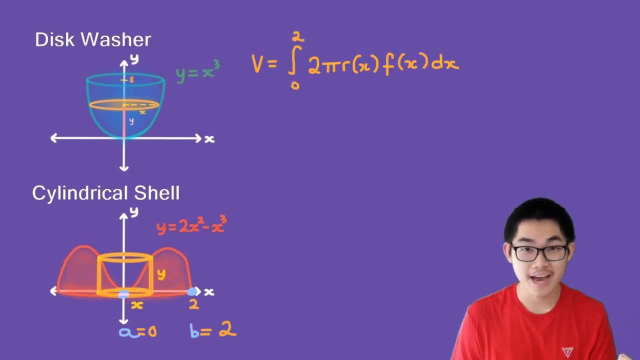 the second step is to find the radius and the height so looking at this shell we know that 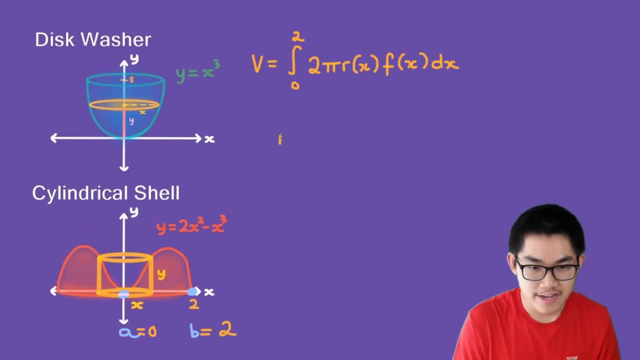 the radius is just x from here to here so the radius r of x is equal to x now how about the height f of x the height is just y so f of x is equal to y and we know that y is equal to this 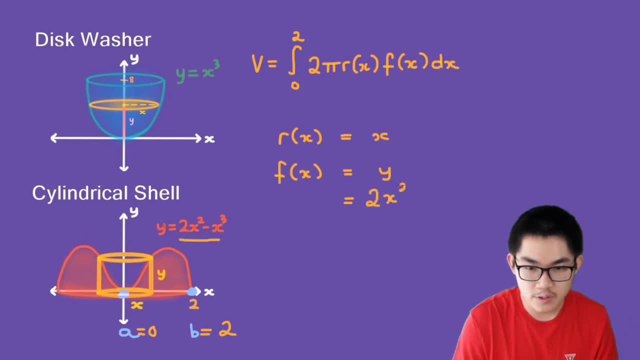 right here so that's going to be two times x to the power of two minus x to the power of three 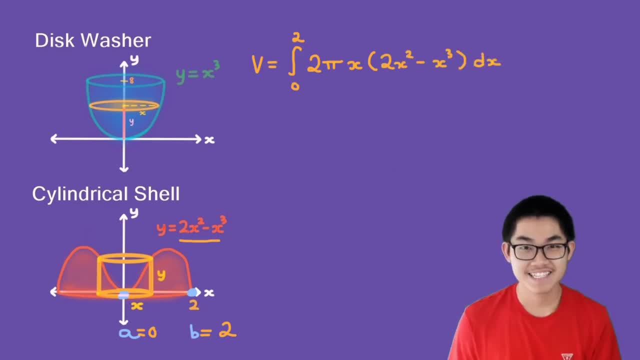 step number three and the last step is to evaluate this integral so since two pi is just a constant we can move it outside of the integral so we're going to get two times pi times the integral from zero to two and x times this we're going to get two times x to the power of three minus x to the power of four dx and this is the same as you're going to get two times x to the power of three minus x to the power of four dx